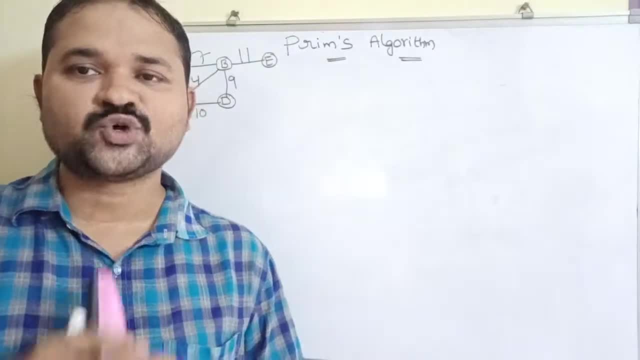 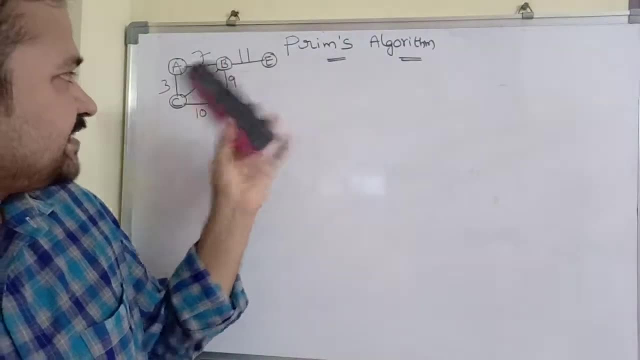 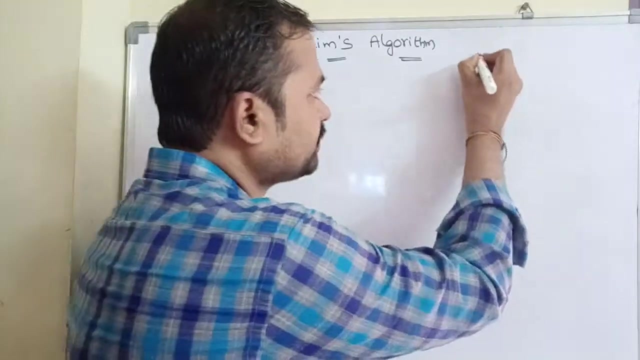 cost than the remaining spanning trees. So now, with the help of the Prim's algorithm, we have to construct minimum cost spanning tree for this graph. First let us see the algorithm. Now let us see the Prim's algorithm. The first step is start with any vertex of the graph. 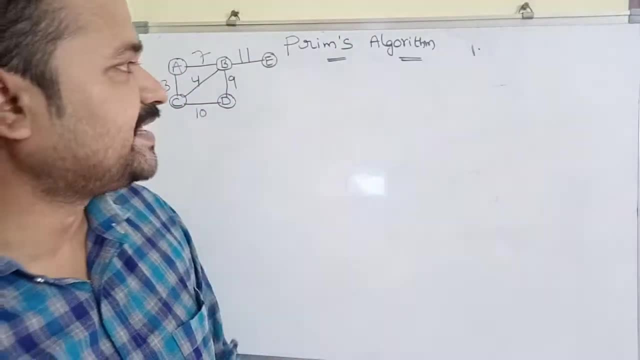 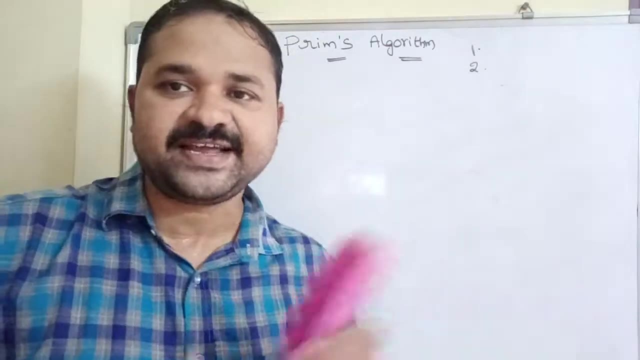 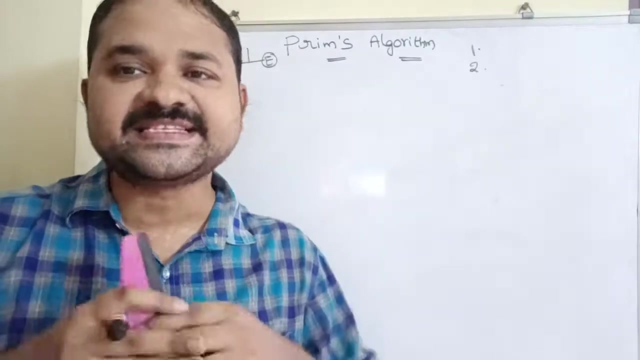 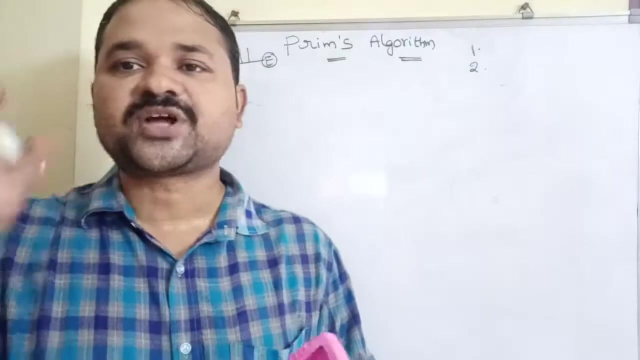 So we can start with any vertex from the given graph. The second step is find the edges associated with that vertex and add minimum cost edge to the spanning tree If it is not forming any cycle, suppose. if it is forming any cycle, then discard that edge. So what is the first step? Start with any vertex of the graph. 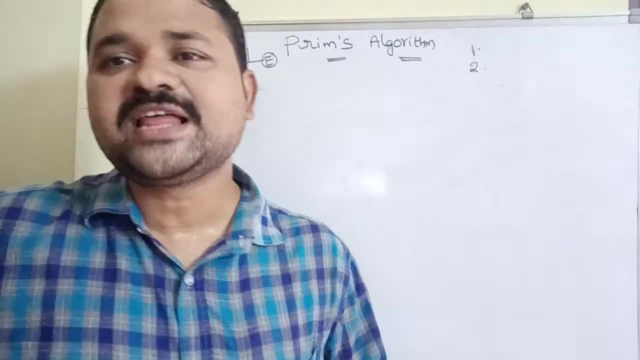 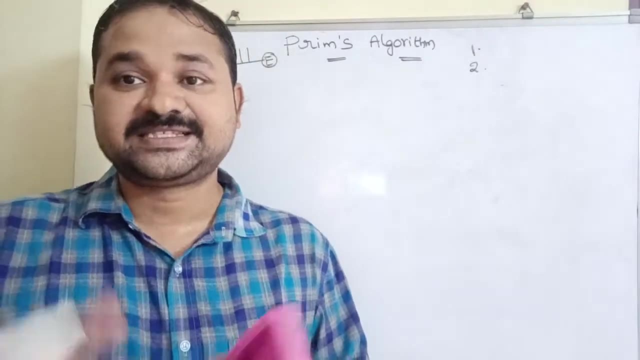 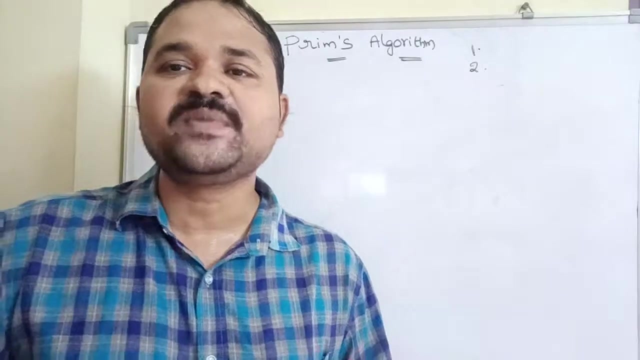 Second step: we have to find out all the edges associated with that vertex and from the available edges, select the minimum cost edge and add that edge to the tree. If it is not forming any cycle, then discard that edge. So what is the first step? Start with any vertex of the graph. 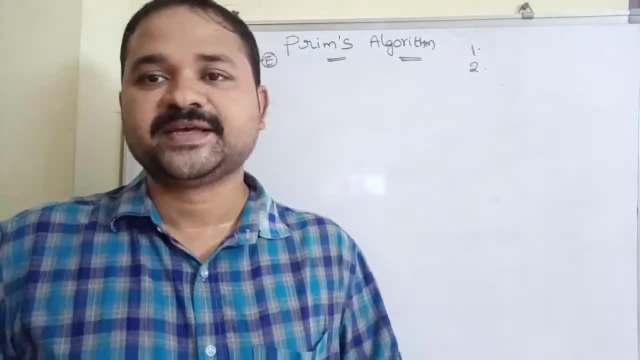 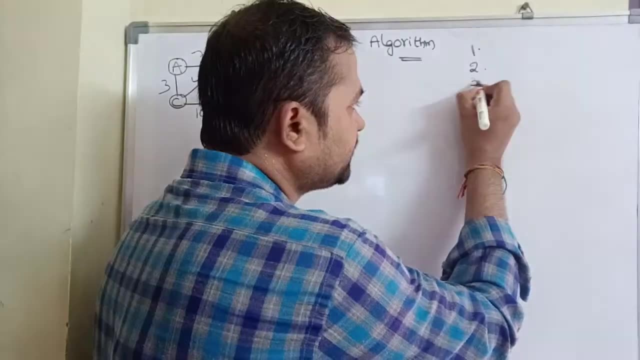 If it is not forming any cycle, suppose by adding that edge. if a cycle forms, then we have to discard that edge. So that is the second step. Next third step, we have to repeat step 2 till all the vertices are covered. 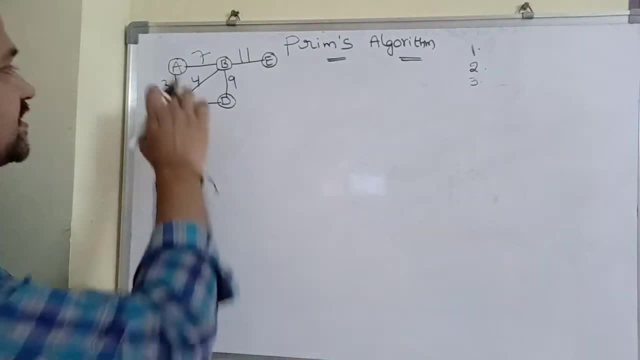 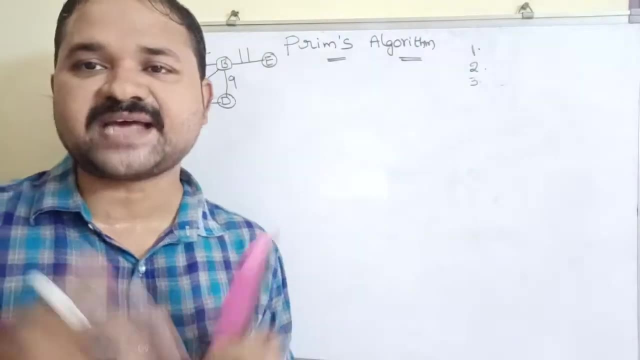 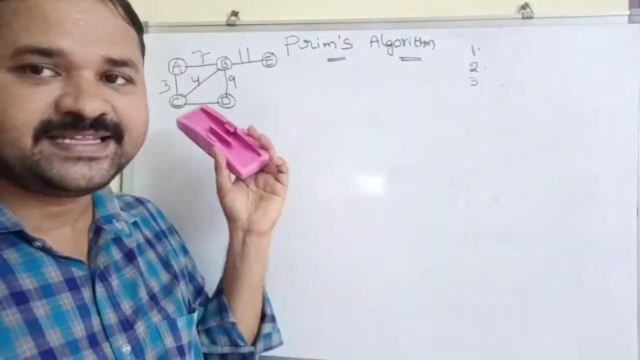 Now this graph contains how many vertices? So 1,, 2,, 3,, 4,, 5.. So this graph contains 5 vertices. We know that spanning tree should satisfy 3 properties. The first property is spanning tree should contain all the vertices of the graph here. the graph contains five vertices. 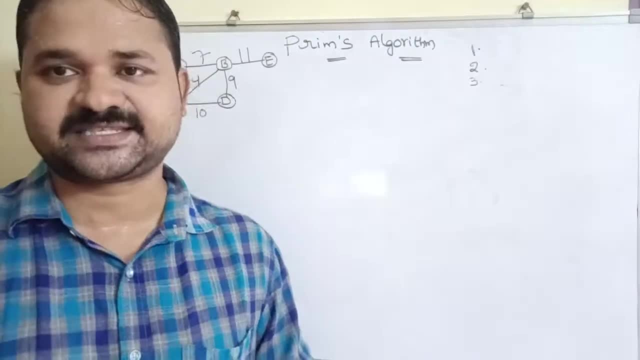 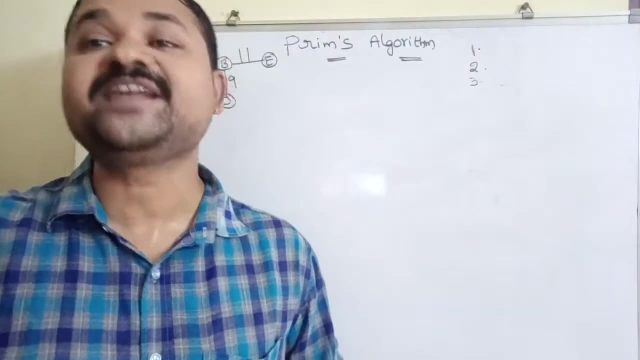 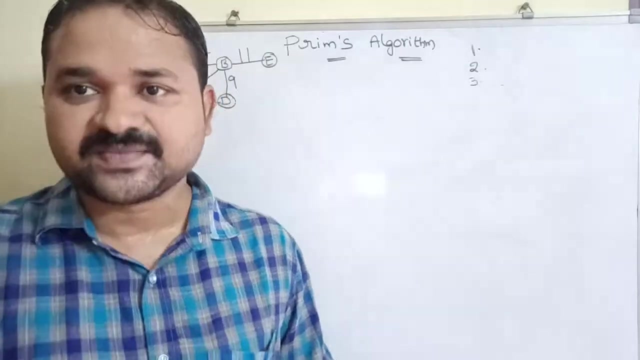 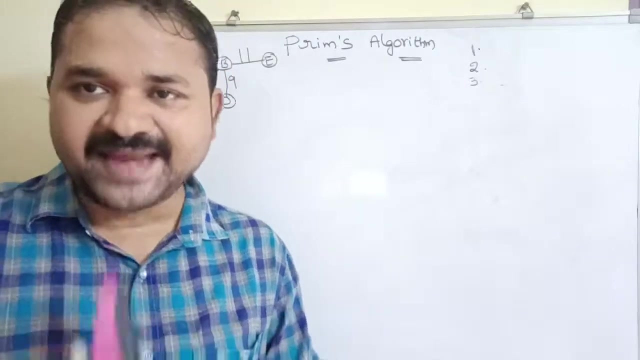 so the spanning tree should also contains five vertices. the second property is: if the graph contains n vertices, then the spanning tree should contain n minus one edges. here the graph contains five vertices, so spanning tree should contain five minus one edges. so five minus one means four. so spanning tree should need to contain four edges. and the third property is spanning tree. 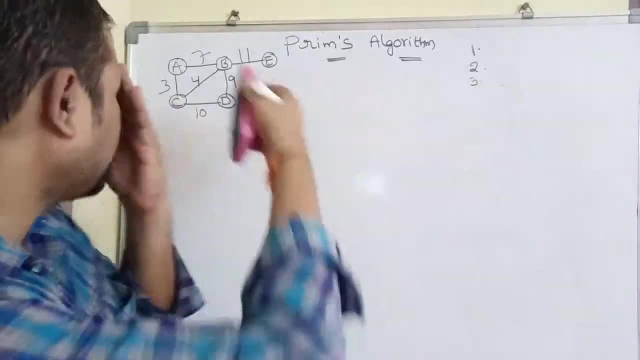 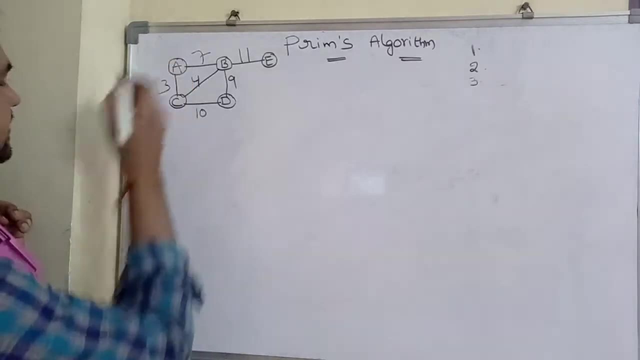 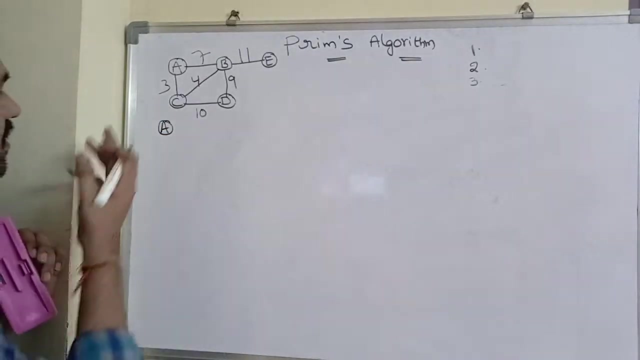 should not contain any cycle. okay, let us do the. let us solve this problem with the help of that algorithm. so we have to select any vertex as the starting vertex. let us start with a vertex. so let us start with a vertex. so let a be the starting vertex. so we have to find out all the 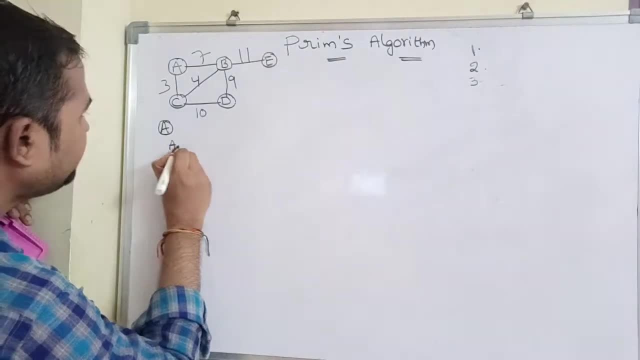 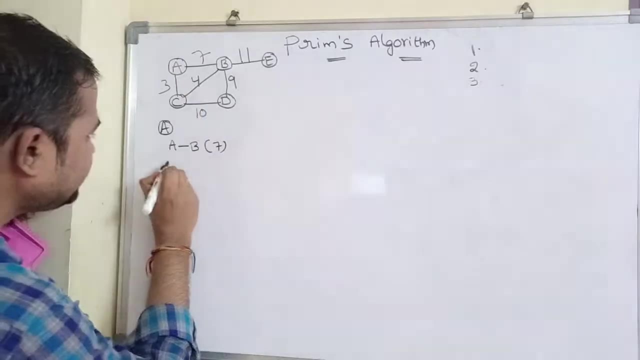 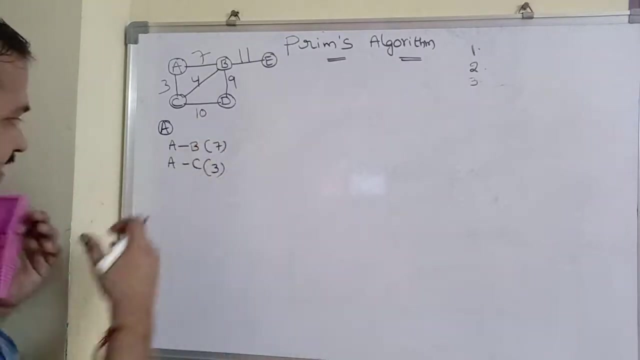 edges associated with a. so what are the edges associated with a? so we have to find out all the images. the first edge is a to b. the cast of this edge is set it, and then extra to c, the past of the sería 3. okay, so what we have to do now, out of all these two edges, a to c has least. 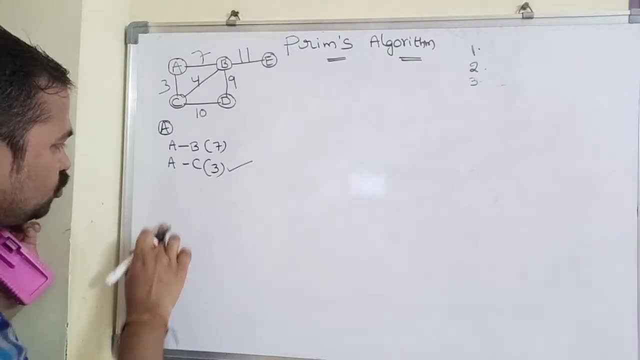 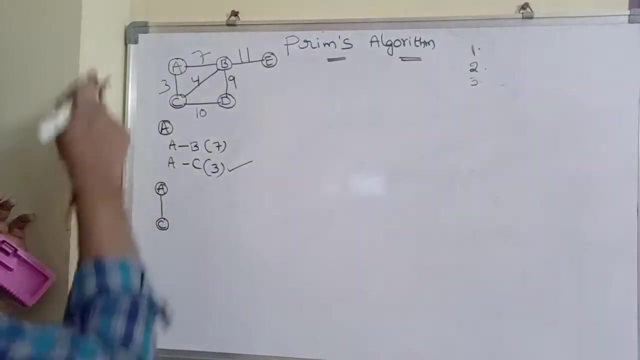 cost edge. so we have to add this edge to the spanning tree if it is not forming any cycle. so initially it is empty. so what we can do? so we can add c, so we add c to the spanning tree 3. Why? Because by adding this edge, cycle does not form. So what is the cost of this edge 3.? 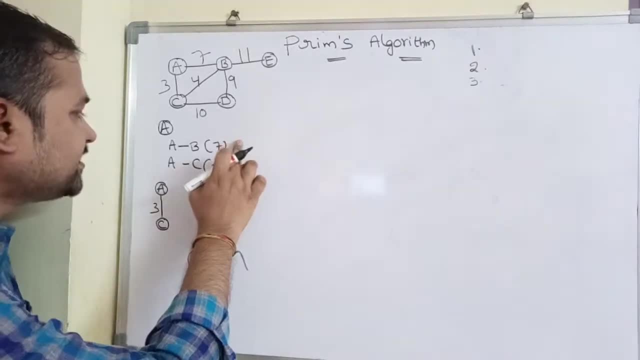 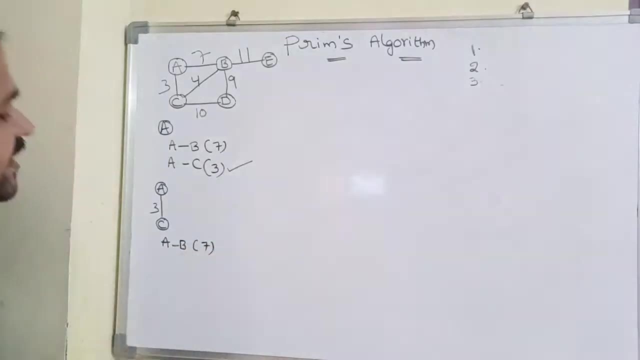 Next, A to C is included. So what are the remaining edges? So we have only one edge, that is A to B. So A to B. what is the cost of this edge 7.. So this is the remaining edge. 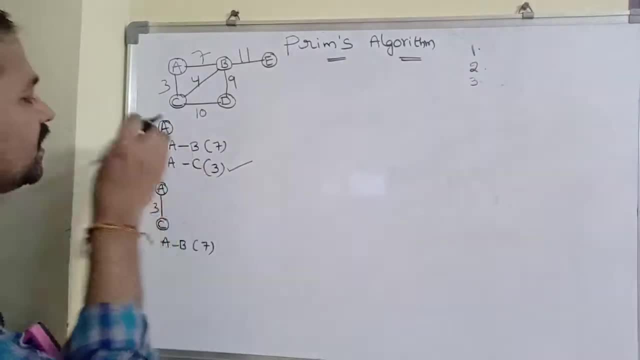 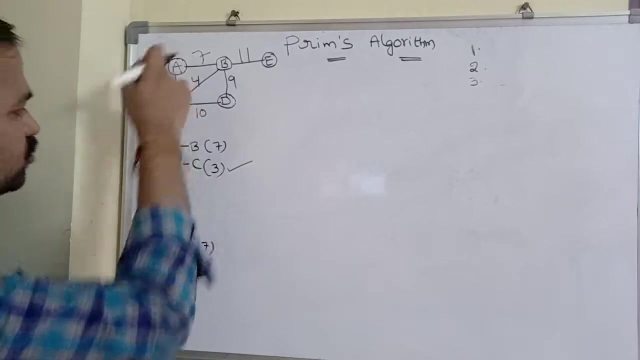 Then, after that, what is the new vertex that we added here, C? So C is the new vertex that we added here. So find all the edges associated with C. So what are the edges associated with C? We have C to A, but that is already included. So what are the other edges, C to B? 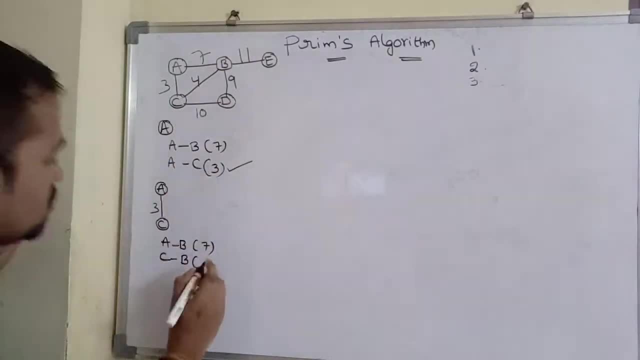 C to B. So the cost of this edge is 4.. And the next edge is C to D. The cost of this edge is 10.. The cost of this edge is 10.. So, out of all these three edges, 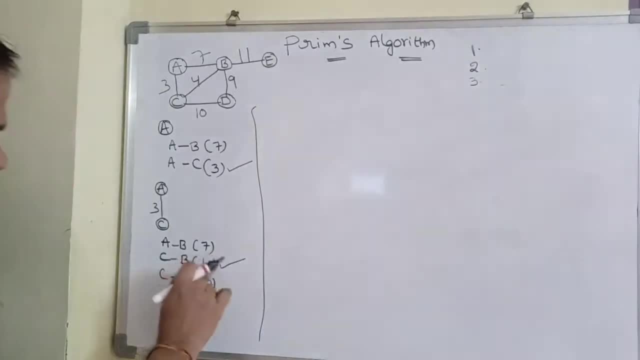 which edge has been added? C to D. So, out of all these three edges, which edge has been added? Minimum cost? C to B, 4. This is the minimum cost. So by adding this edge here, we have B here. 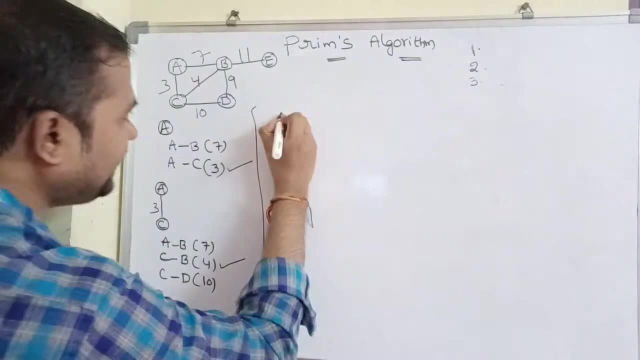 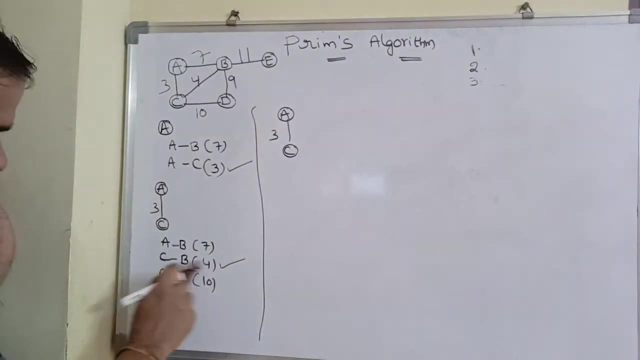 So by adding this edge cycle does not form. So we can add this vertex. So A to C. what is the cost here? 3. Next, the minimum cost here is 4. So we add C to B. So this is the edge here. 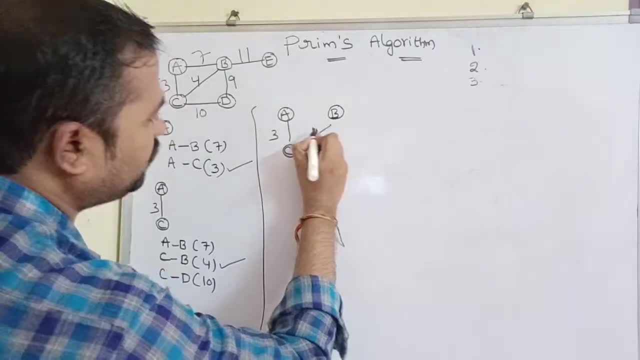 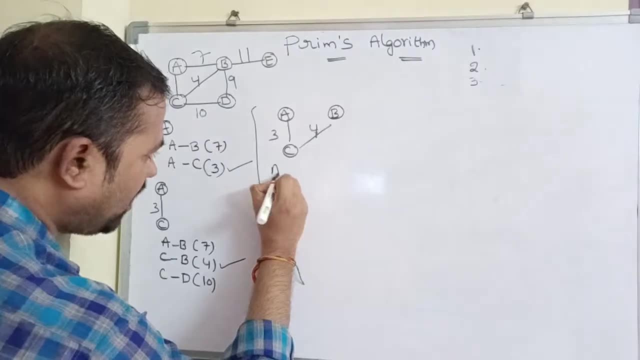 So C to B. So we add this edge. So what is the cost here? 4 is the cost here. What is the cost? 4 is the cost here. Now, what are the remaining edges here? We have two remaining edges. First one is A to B. 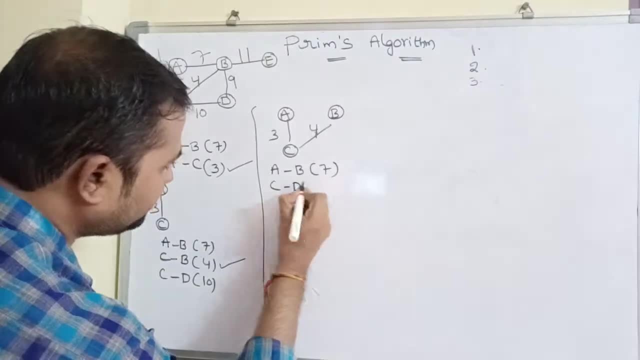 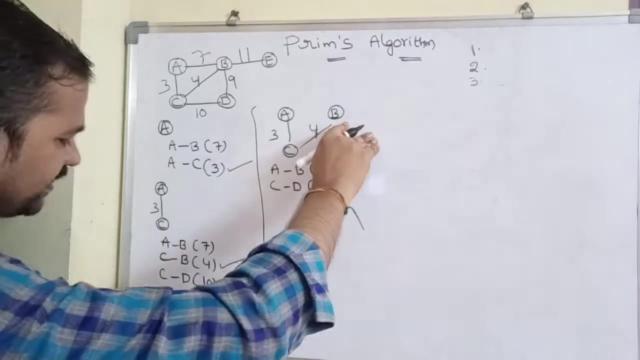 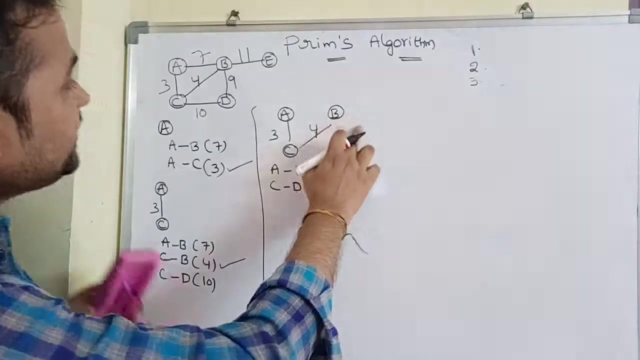 The cost of this edge is 7.. Next one is C to D. The cost of this edge is 10.. Next, what are the edges that are associated with the new vertex? So what is the new vertex that is added here? B? So we have to find out the edges associated with B here. So what are the? 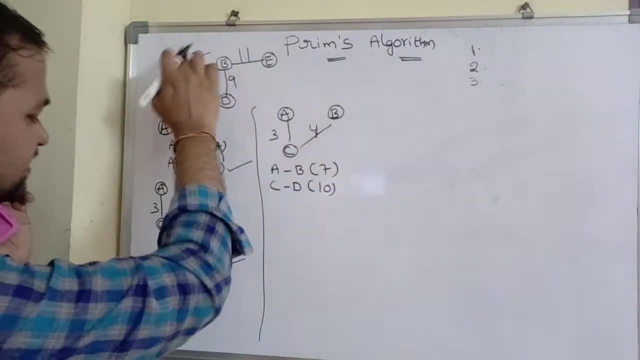 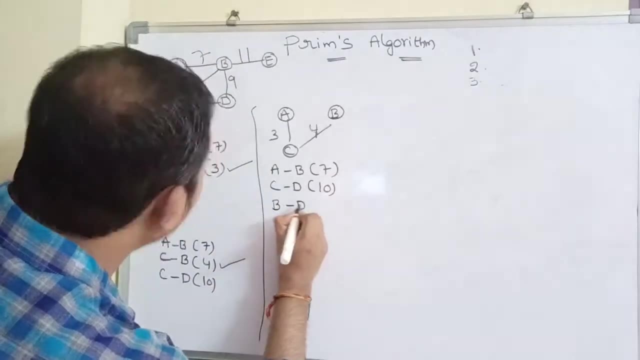 edges associated with B. We have three edges. First one is A to B. That is already included. So next one is B to D, So that is not included. So we add this edge, So B to D. What is the? 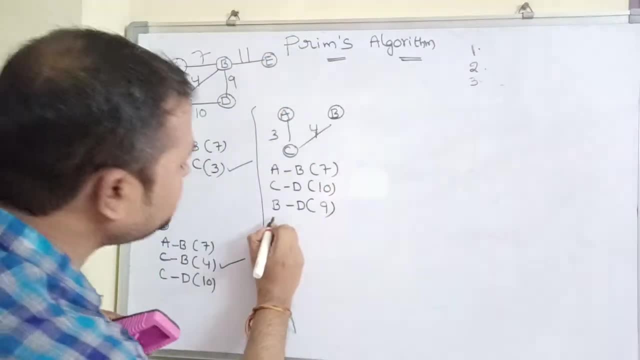 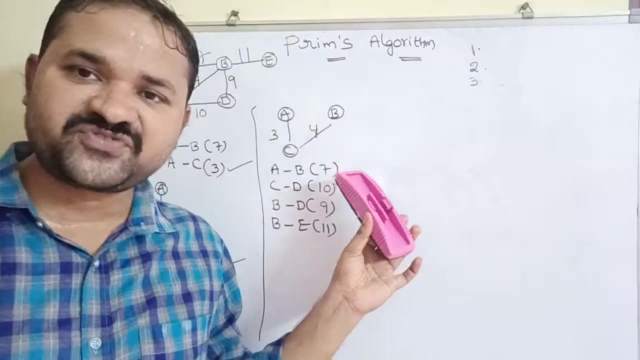 cost of this edge: 9.. Next, we have one more edge, That is B to E. The cost of this edge is 11.. So, out of 7,, 10,, 9 and 11.. So which is the smaller value? So 7 is the smaller value. 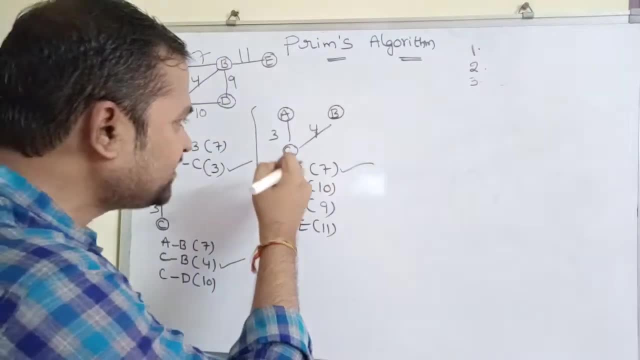 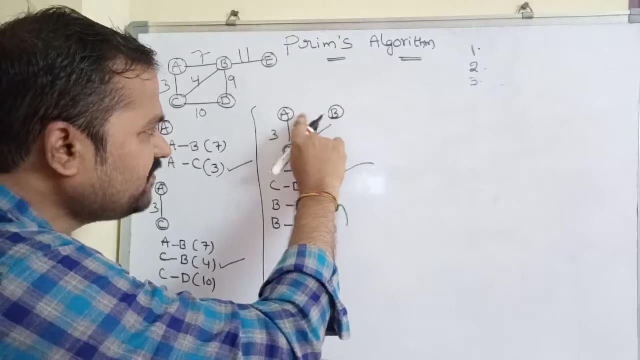 So we have to find out whether by adding this edge, whether a cycle reforms or not. A to B: So if we add A to B here, then what will happen? A cycle will be formed, So we have to discard this. 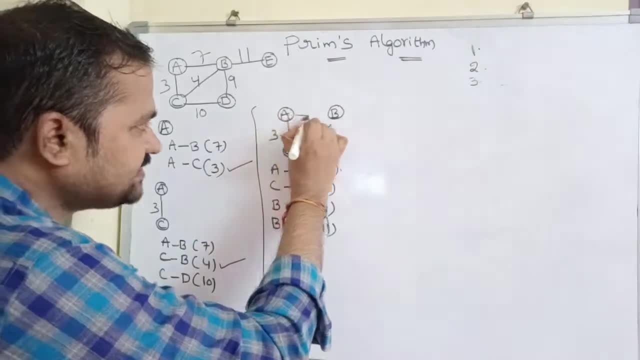 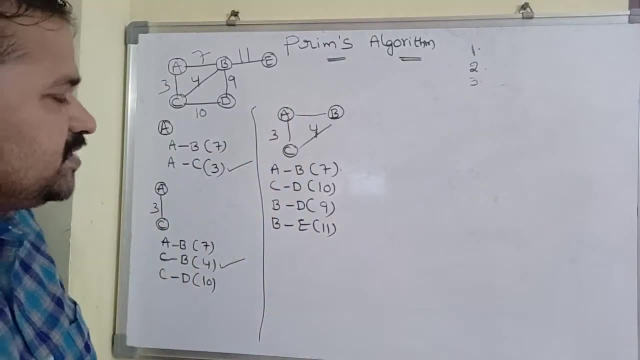 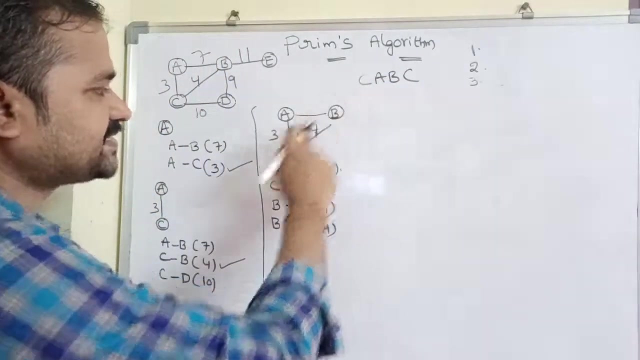 edge, Because if we add this edge, then what will happen? This is a cycle. What is a cycle? A cycle means it contains a path in which the starting vertex and the destination vertex are the same. If you take this path, C, A, B, C, So here C is the source vertex, So from C. 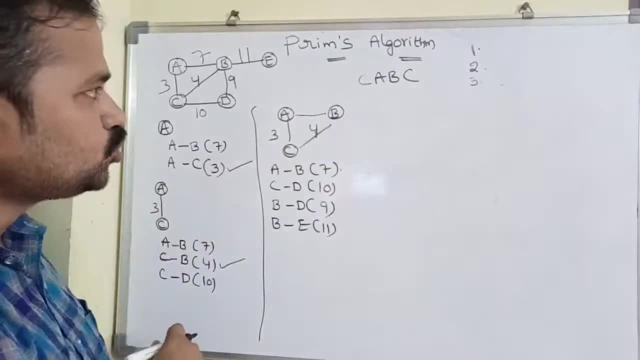 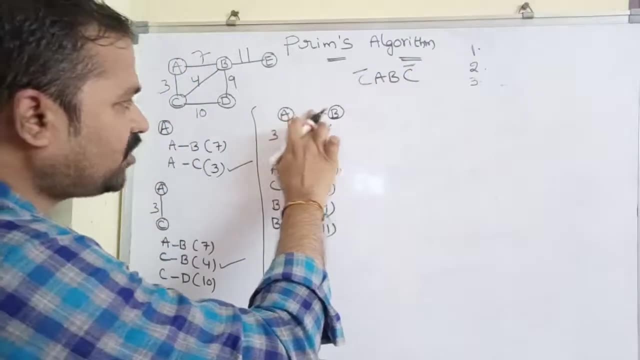 we can go to A, From A we can go to B, From B we can go to C. So here this is a path in which the starting vertex and the destination vertex are the same, So we should not add A- B. 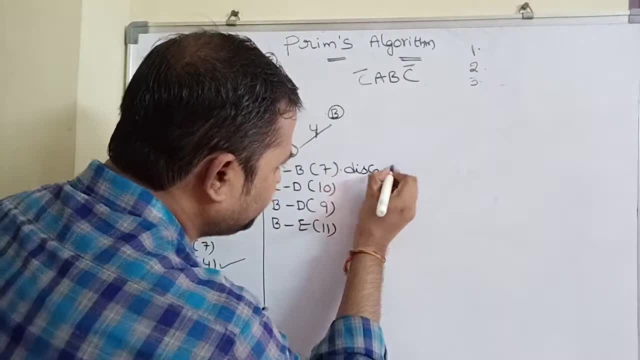 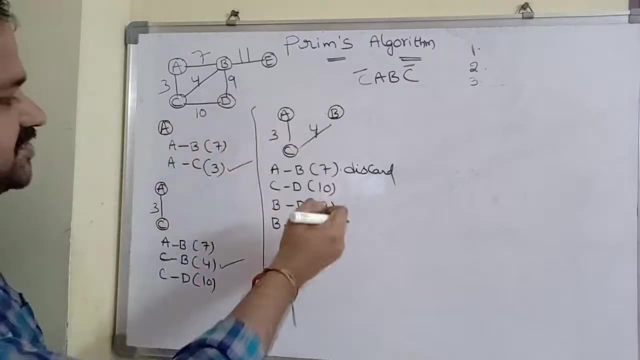 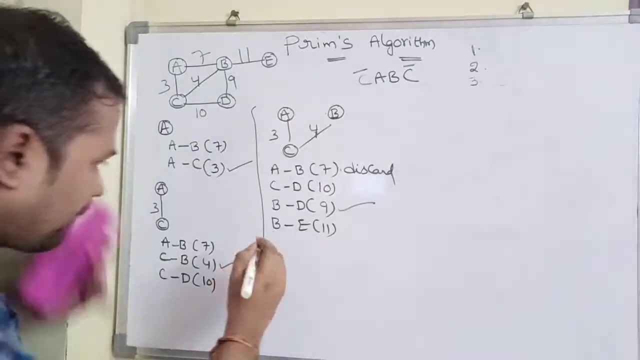 So discard this edge. So discard this edge. So what is the next minimum value? 9 is the next minimum value. So by adding this edge, is there any possibility of psychic? Here we have G, So there is no psychic. So add this edge to the graph. So what is the previous 3?? So A to C. 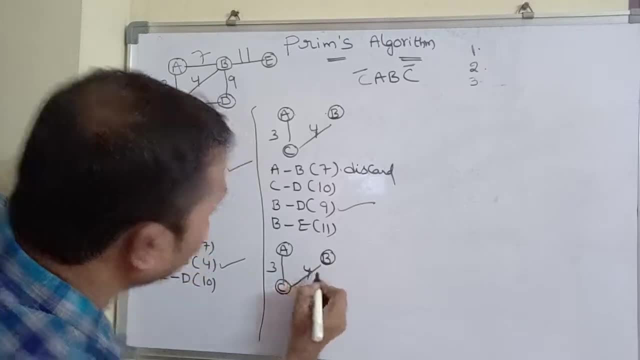 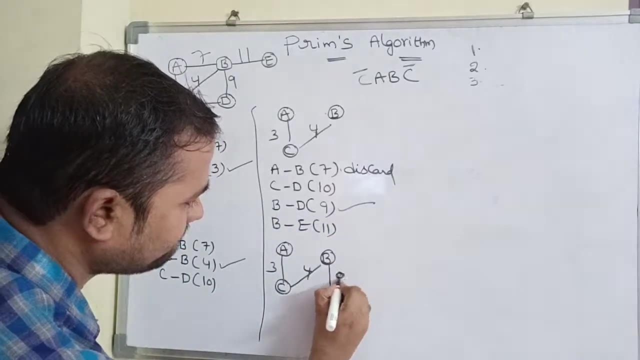 next one, C to B. What is the cast here? 4 here Now we have to add dH to this, Styleинки. So what is the cast here? 9.. 9 is the cast. So what are the remaining edges now? 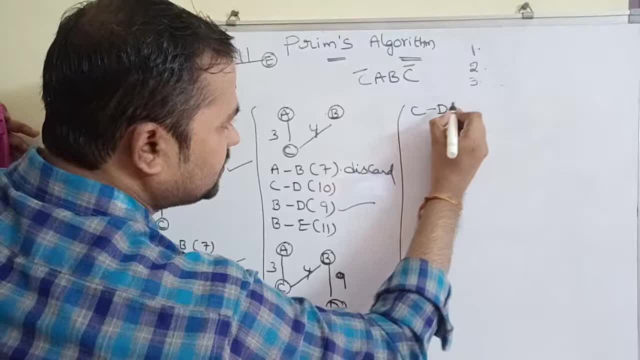 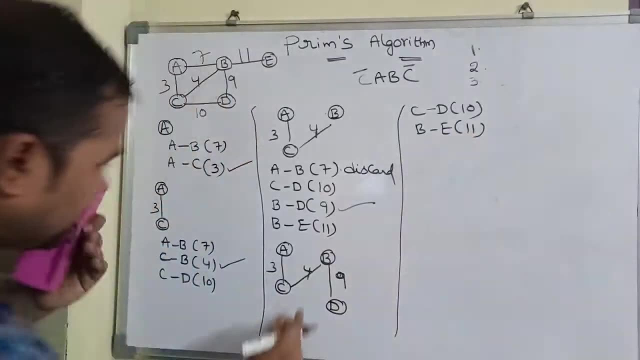 C to D. we have two remaining edges: C to D. the cast of this edge is 10.. Next one, B to E: the cast of this edge is 11.. So what is the new edge that is added here D? So we have to find. 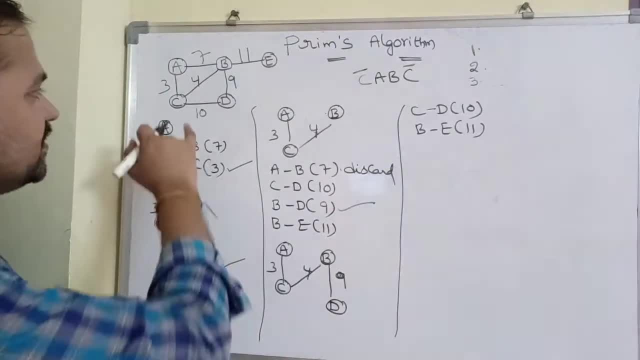 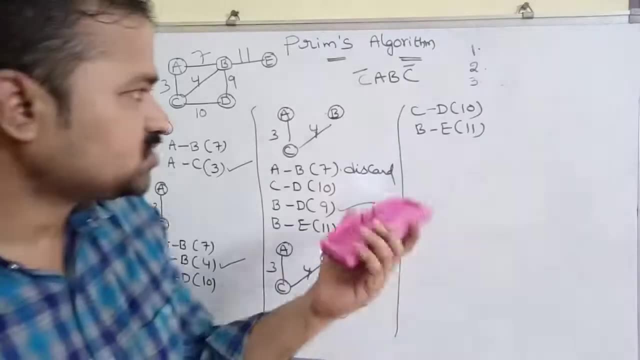 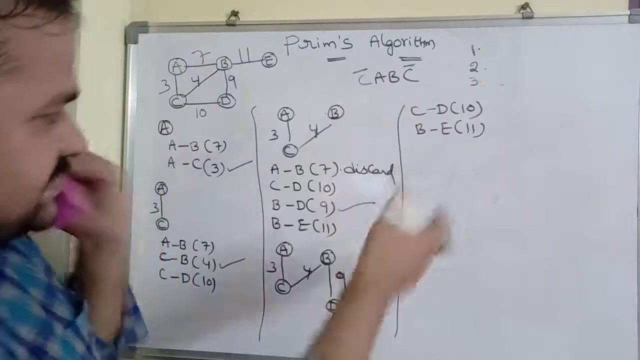 edges that are associated with d. so what are the edges here? we have two edges, c to d, already included, next to b to d. that is also already included. so there is no x, there is new h, there is no new h. so we have to check whether is there is any possibility to add these edges or not. so 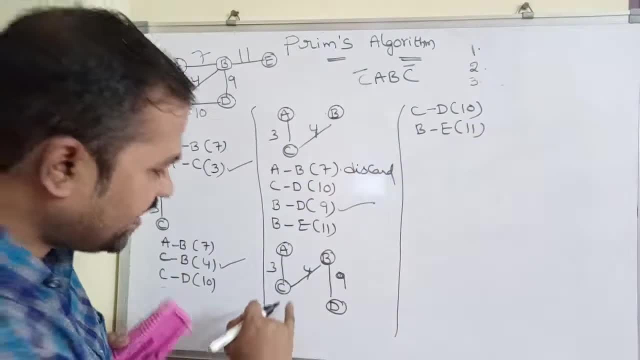 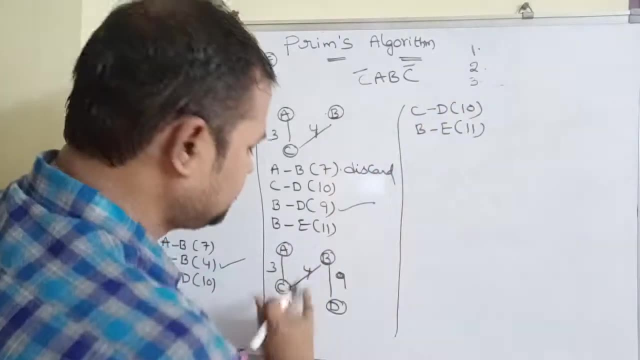 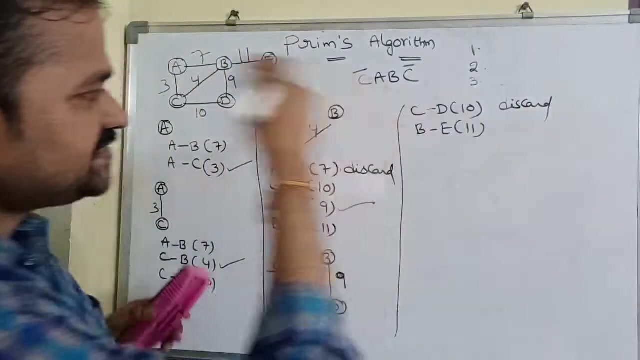 out of 10 and 11, which is the minimum value. 10 is the minimum value. but if we add c, but if we connect c and d, then what will happen? a cycle will be formed. c to d. if we add this one, what will happen? a cycle will be formed. so we have to discard this h. so what is the last edge here? b to e, here. 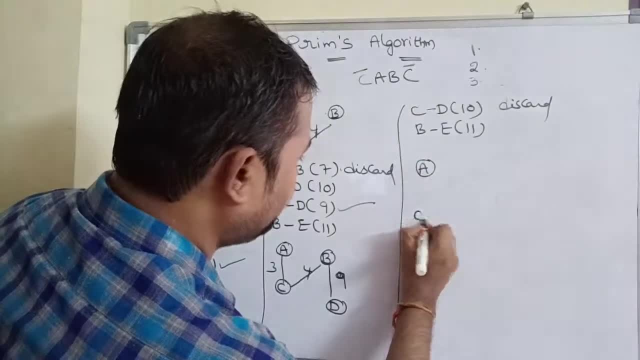 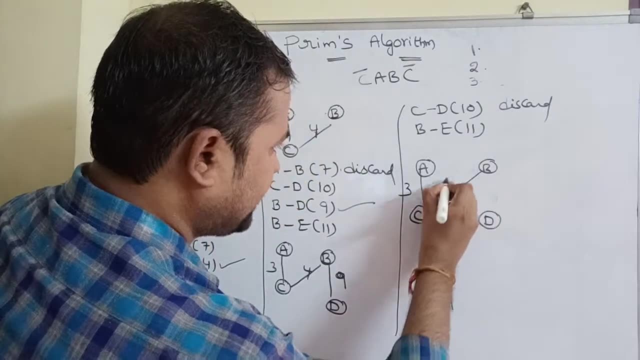 we have e. so by adding this h, no cycle will be formed. so a to c. next here we have b, here we have t. here the cost is 3, here the cost is 4, here the cost is 9. so b to e, what is the cost here? 11. 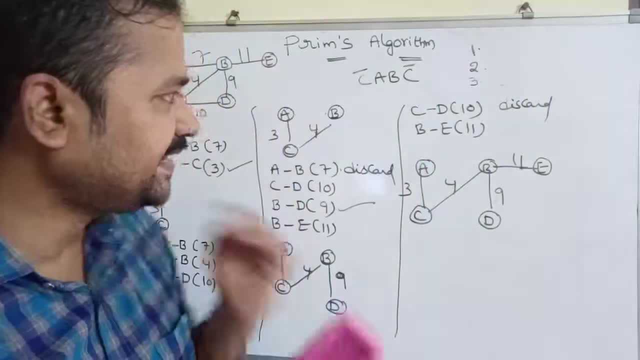 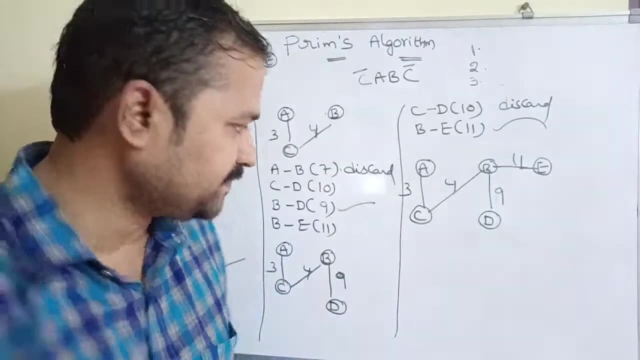 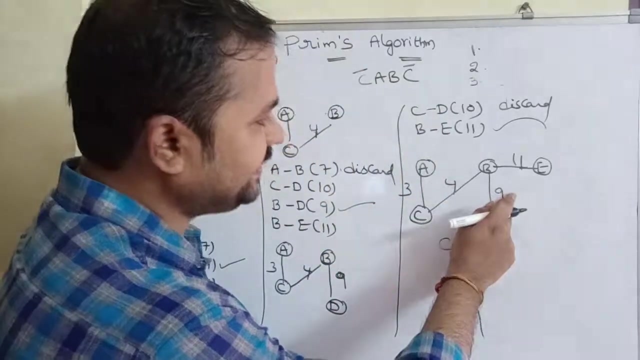 okay, so all the vertices are covered. okay, so this edge is included. okay, so this is the minimum cost spanning tree that is obtained with the help of the prim cell algorithm. and let us calculate the cost of this spanning tree. so 3, 3 plus 4, 7, 7 plus 9, 16, 16 plus 11, 27, so 27, 11 plus 9, 20, 24 and 3. 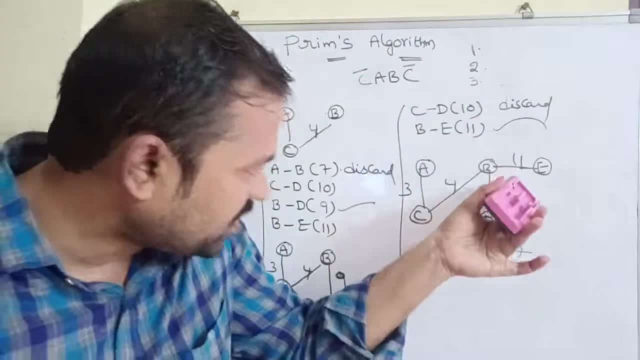 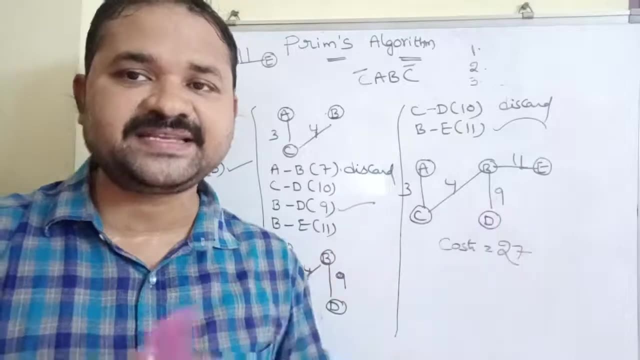 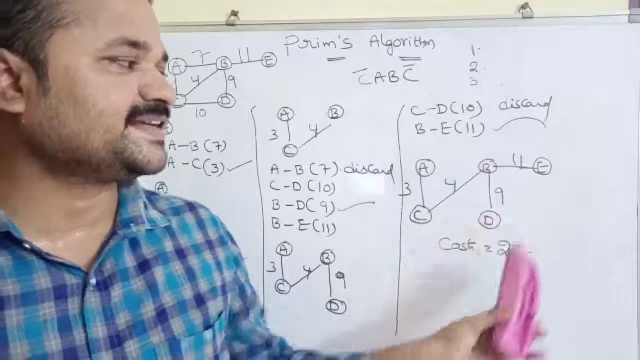 27. let us check whether this minimum cost spanning tree it is satisfying our spanning tree properties or not. so what is the first property for a spanning tree? it should contain all the vertices of the graph. so our graph contains five vertices, whereas our spanning tree contains five vertices. so the first property is satisfying. second,